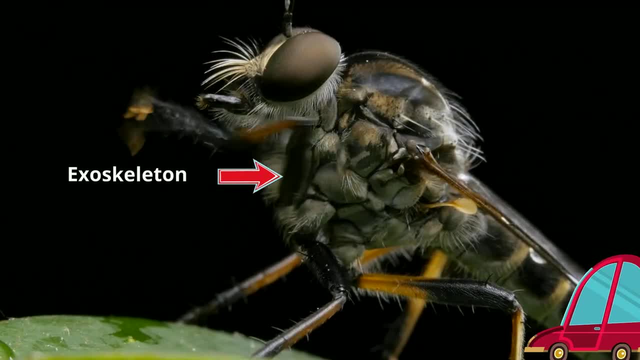 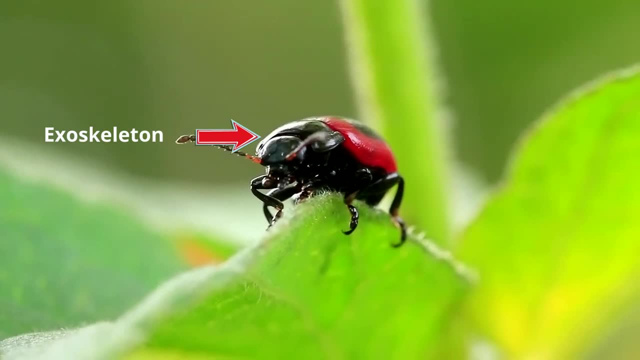 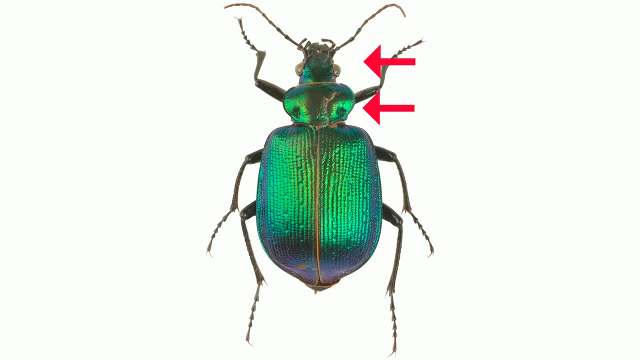 called an exoskeleton. Think of an exoskeleton like the outer body of a car. The job of the exoskeleton is to give the arthropod support and protection. Arthropods also are composed of segments. For example, an insect has a head, thorax and abdomen, or three body segments. 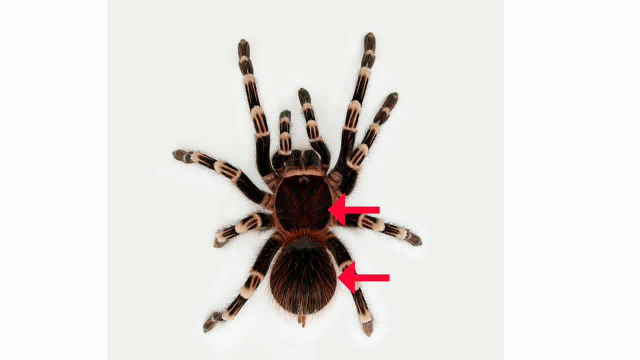 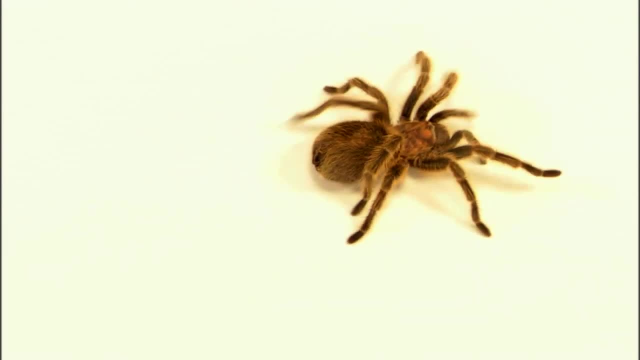 Spiders have two body segments and centipedes have 20 or more segments. Arthropods are famous for their appendages, For example, the legs of a spider, the antennae of wasp. What makes arthropods unique is that the appendages are so large that they can 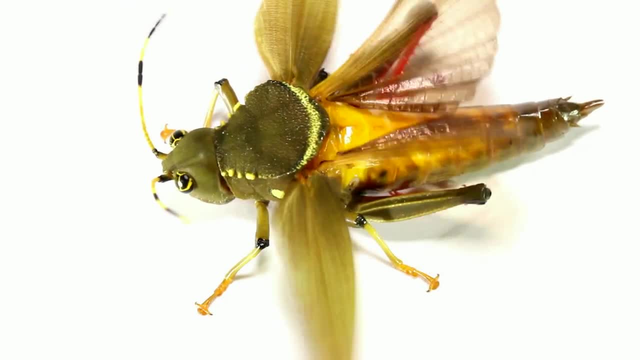 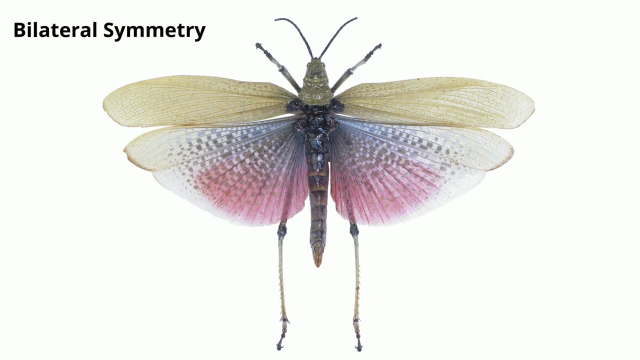 have many joints. These joints allow the arthropod to move, jump or even fly. Arthropods have bilateral symmetry: They look the same on each side. If you run a line from the top to the bottom of an arthropod, it will look the same on each side. 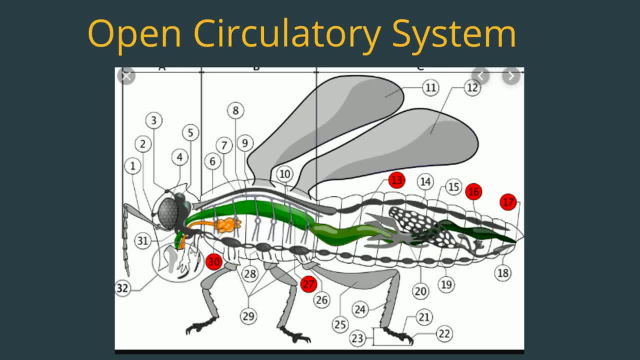 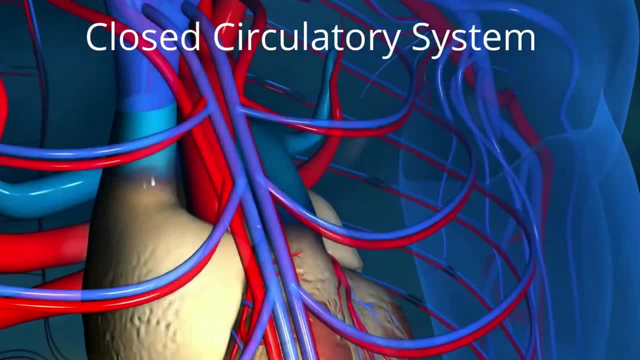 Arthropods have an open circulatory system. An open circulatory system uses cavities called sinuses that move the blood around the body. Closed system circulation, which will cause the blood to move around the body, will cause the blood to move around the body. 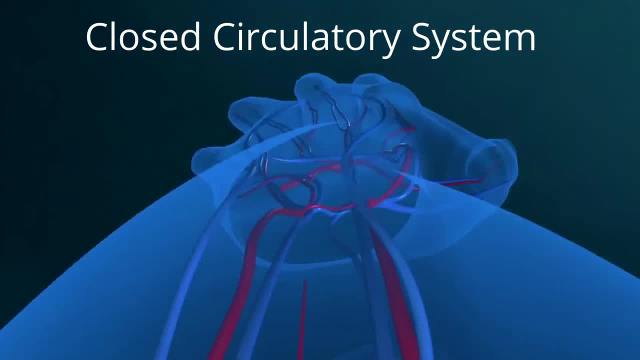 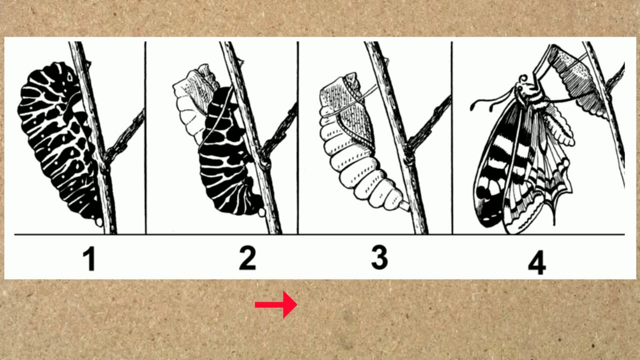 Closed system. circulation which we have uses veins and capillaries and arteries in order to move blood throughout the body. Many arthropods carry out metamorphosis, which is the process of transforming from an immature form to an adult in two or more distinct 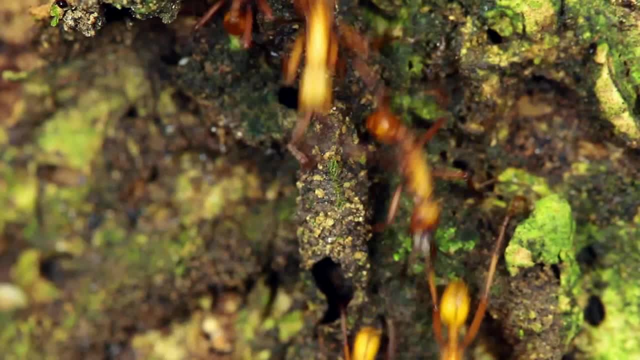 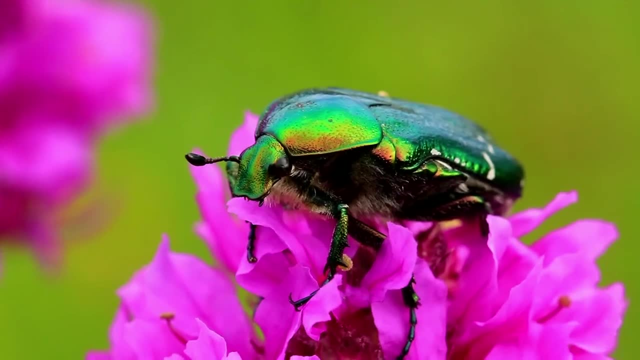 stages. Arthropods are everywhere. They are the largest animal phylum. There are over 1 million species of arthropods and a huge variety of tasks. Here are four sub-phyla of arthropods to give you an example of some of these. Arthropods are the largest animal phylum. They are the largest animal. 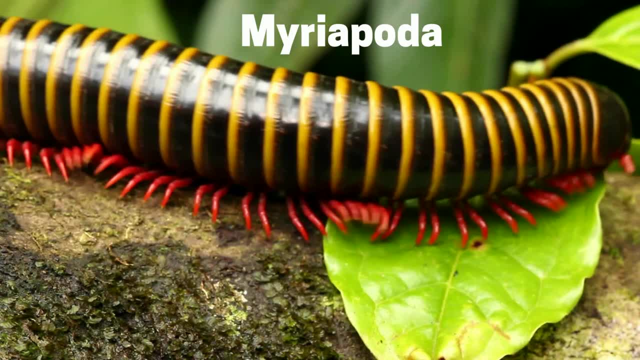 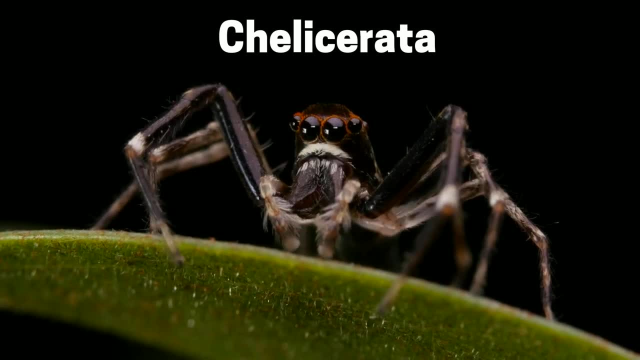 that has been in the world since the beginning of the human race. They are the largest animal that has been in the world since the beginning of the human race: Myriapoda, which includes centipedes and millipedes. Chelocerata, which includes spiders, scorpions and ticks. Crustacea. 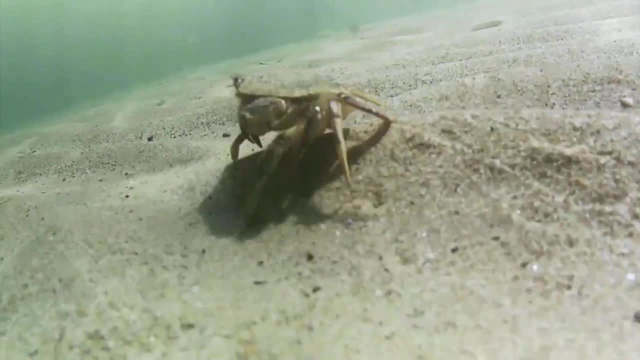 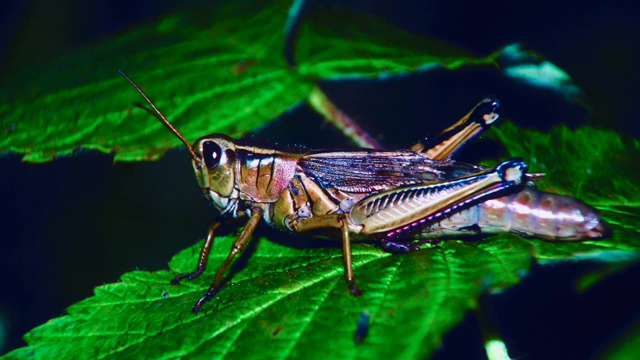 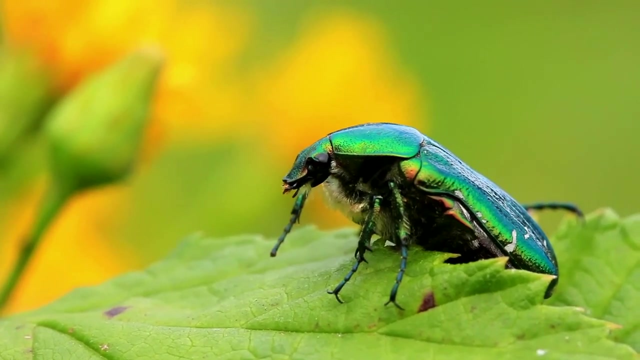 which includes lobsters, crab and shrimp, And hexapoda, which includes ants, flies and grasshoppers. So there we go. if you would like to know more about arthropods, This playlist will help and, as always, thanks for watching. and MooMooMath uploads a new. 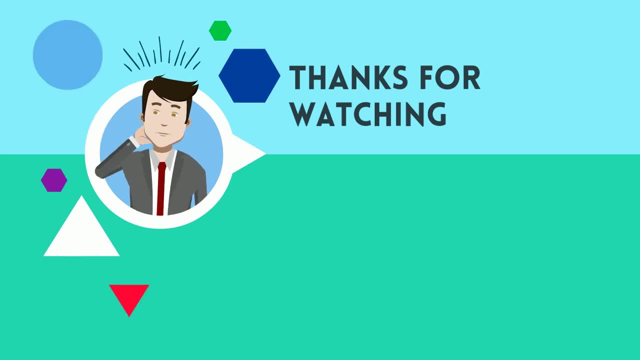 math or science video everyday. Please subscribe and share.